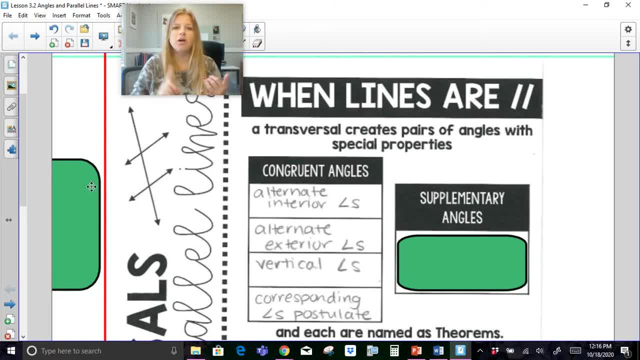 corresponding angles are congruent And we use alternate exterior, interior angles theorem, alternate exterior Angles theorem, vertical angles theorem, We can call it the corresponding angles theorem or we can call it the corresponding angles postulate, just the names for them. But we 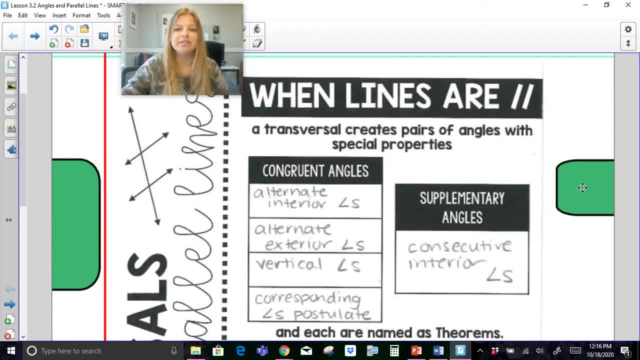 have one other special situation that happens: Our consecutive interior angles are supplementary. So alternate exterior are congruent, Alternate interiors are congruent. Corresponding angles are congruent. Vertical angles are always congruent, But now consecutive interiors. so this pair of angles and this pair of angles, they are actually supplementary. They make 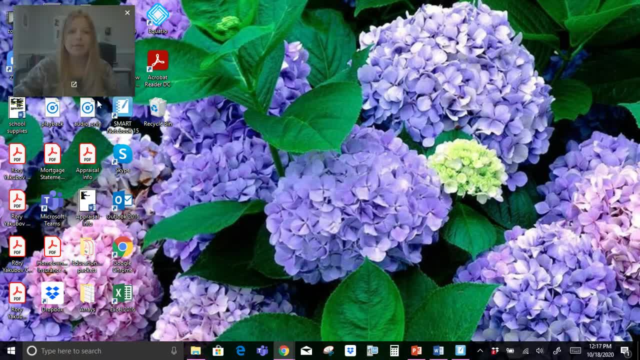 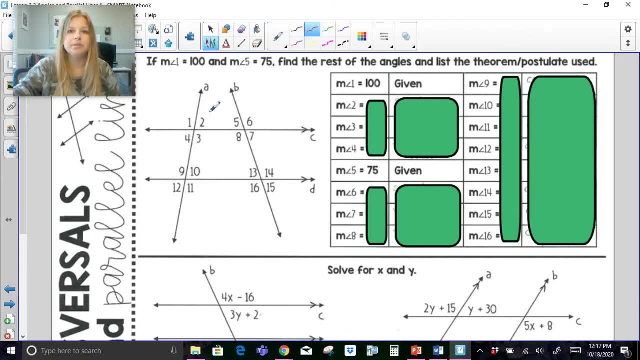 180 degrees. So we're going to take a look at this diagram here. Sorry about that. So it says here: if the measure of angle one is 100, so I'm just going to label that- and the measure of angle five is 75.. Find the rest of the angles and list the theorem or. 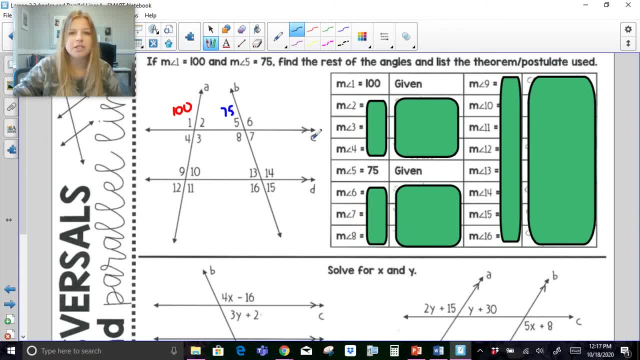 postulate used. So here I have this notation, guys, Take a look. That's a lot of times, but line C and line D are parallel to each other. When you have that little extra arrow on a line, it indicates that the lines are parallel, which means I have two different transversals. I have 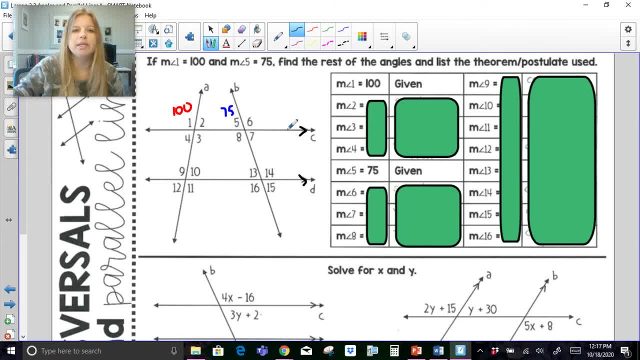 transversal A and transversal B. So we really need to make sure we're very aware of the fact that this line A is a transversal along those angles and transversal B really involves these angles. So notice the angles that deal with the parallel lines should be. 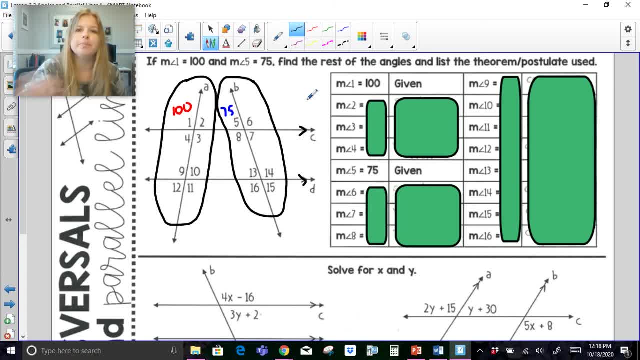 all along the transversal. They're not going to skip over. So the measure of angle one is 100.. We are given that I would then be able to say that the measure of angle two is 80 because they are a linear pair and linear pairs are supplementary to each other. 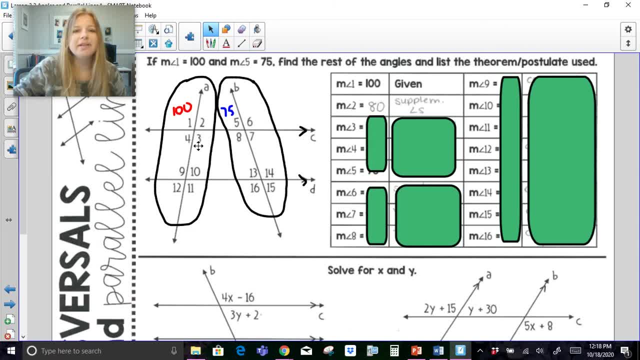 So think about that. Angle two is 80. I could then say: angle three is 100 degrees, because I could either say it's a vertical angles, because of angle one is 100, angle three is also 100, or I could say that since angle two is 80, that's just another pair of. 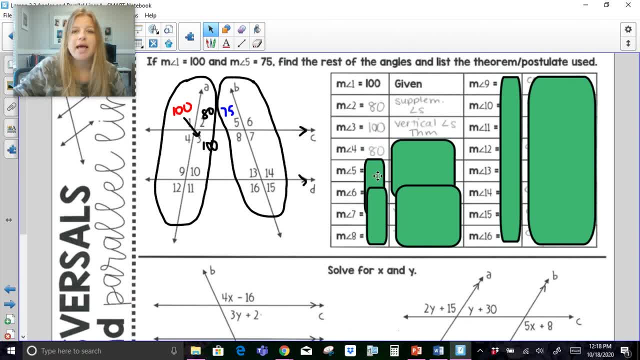 supplementary angles. It's a linear pair. Angle four is then 80 degrees, So I could use kind of the same idea as I can call it by supplementary angles, I could say because of vertical angles. Now let's take a look at angle five. We know that angle five is 75 because we were given that. 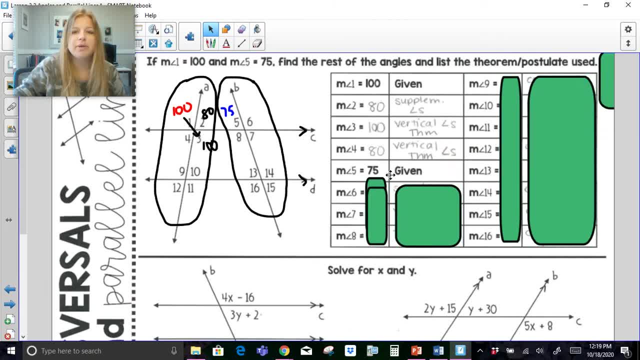 information. But now, if I wanted to figure out the value of the measure of angle three, I could say angle six, I could do the same thing. I could say supplementary, So it has to add up to 180.. So it's 105. And then, going forward, if I know that this is 105, I could use those same properties. 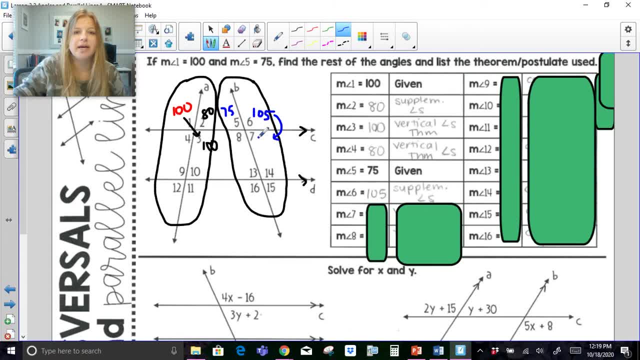 I could say: well, because of supplementary angles, this is 75. And because these are vertical angles, if this is 105, then angle eight is also 105. And so you kind of have different things you could do. You can use your vertical angles to say: if this is 75,. 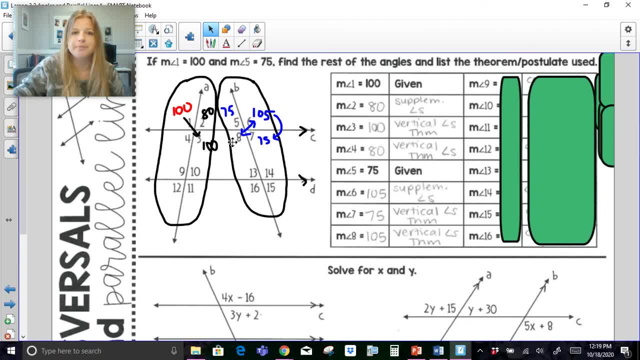 this angle 75, and same thing with 105 and 105. But now jumping down here, okay, so there's going to be a bunch of things that we're going to be able to say and we can really choose. If I said, 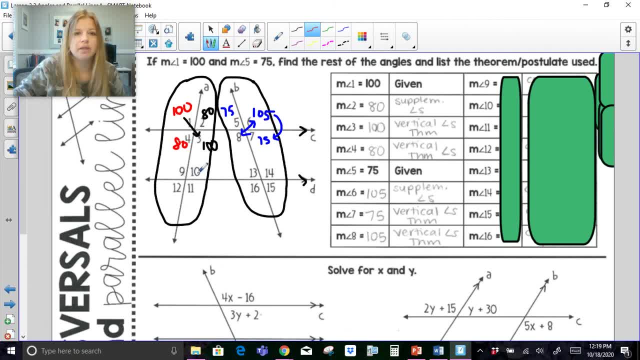 to you what's the measure of angle nine? there's a couple different ways we can look at this. we could say: okay, well, angle one and angle nine or are corresponding. So if angle one is 100 degrees, then angle nine is also 100 degrees. I could say that angle nine is 100 degrees. 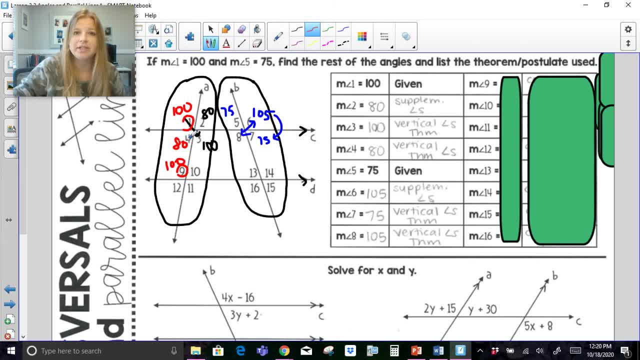 because it's a vertical angle. So if I said to you what's the measure of angle nine, there's a couple different ways we can look at this, because if angle four is 80, and these are consecutive interiors, they have to add up to 180.. So that would be another way to get this 100. So you definitely 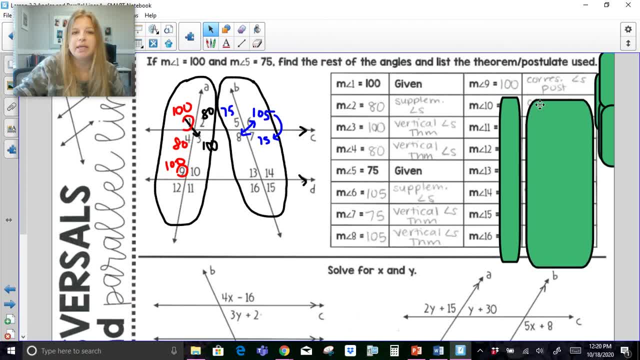 have options. I use corresponding angles, postulate in my answer here. Then for angle 10, there's a couple ways we can do this. We could say: well, angle two corresponds to angle 10.. So if angle two is 80,, then angle 10 is 80. I could use alternate interiors and say: if angle four is 80,. 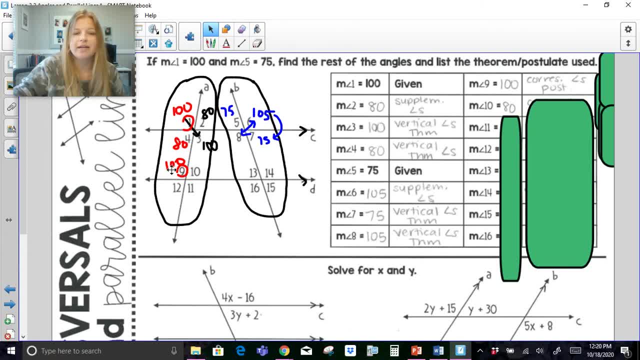 then angle 10 is 80, by alternate interior. Or I could use the fact that they are supplementary to each other, And if angle 100, angle nine is 100, then angle 10 has to be 80. Okay, and the same thing would end up happening for angles 11 and 12.. And you can see I can really 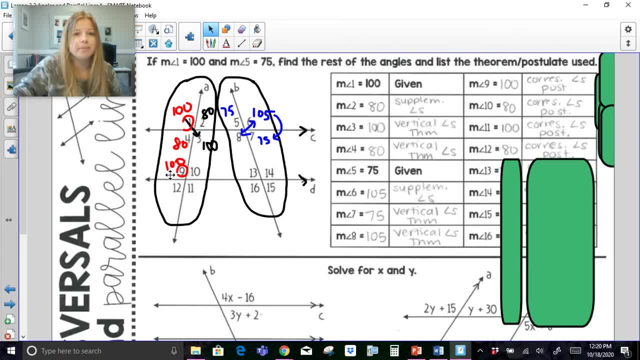 just technically use corresponding angles. postulate for every single one of them. Angle three is 100., So angle 11 is also 100.. Angle four is 80, then angle 12 is also 80. The same thing would happen over here on the right side. So if angle four is 80, then angle 12 is also 80.. The same thing would happen over here on the right side. 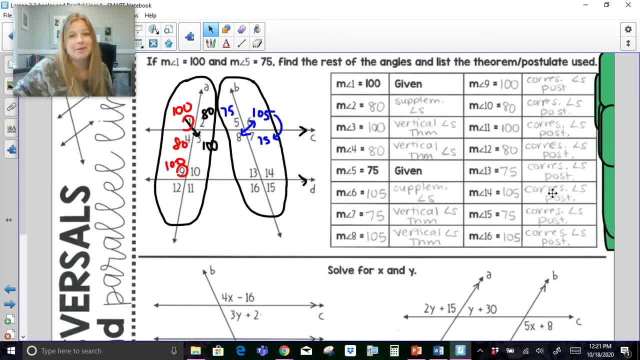 hand side. Again, I just basically almost copied and pasted the corresponding angles postulate for each one of them, But you definitely do have options. So again, if this angle here, number seven, is 75. Well, these are alternate interior, So angle 13 is also 75. And then, because 13 and 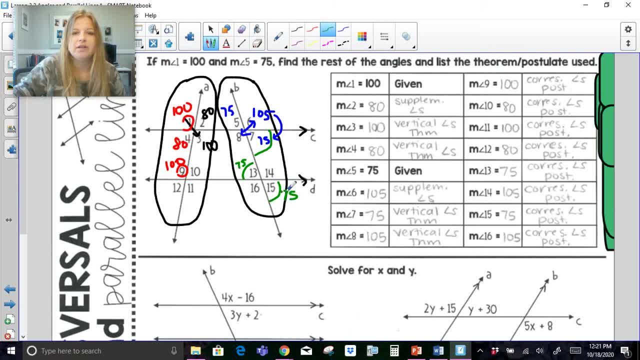 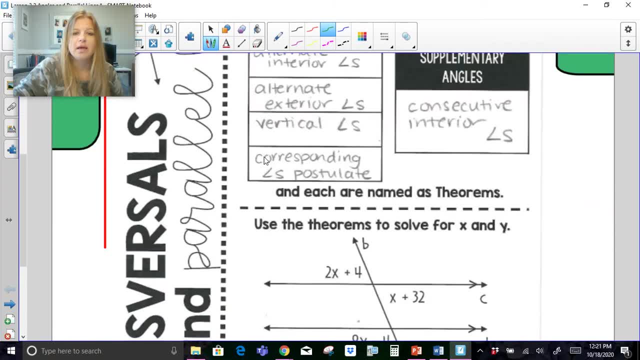 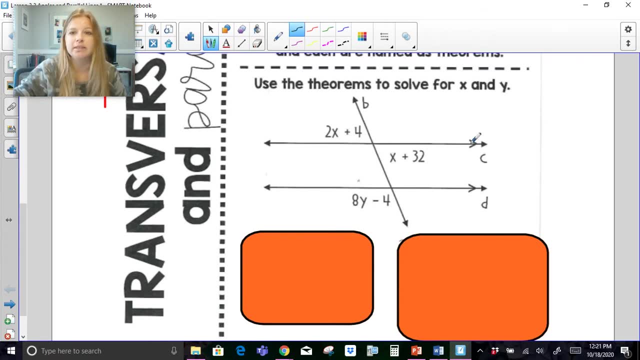 15 are vertical angles. angle 15 is 75. So I could use alternate interiors and then I could use vertical angles. So any of those would be completely fine. The second part of this says: use the theorems. so if angle 12 is 100, then angle 13 is also 75. And then if angle 14 is 100, then angle 15 is also 75. So 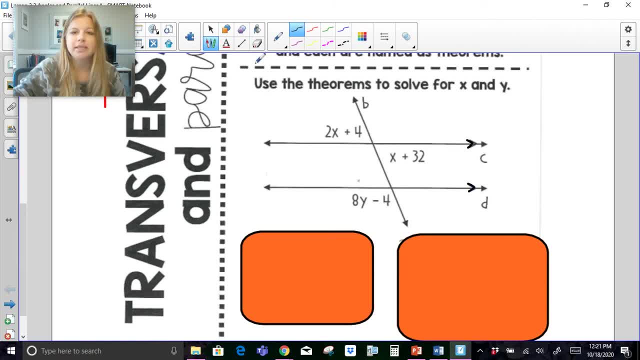 here again, I have a pair of parallel lines. Line C is parallel to line D because I have that extra little indicator there, And let's think about some things that we know. So, first of all, we know that this angle here, where I have two x plus four, has to be equal to x plus 32, because those are 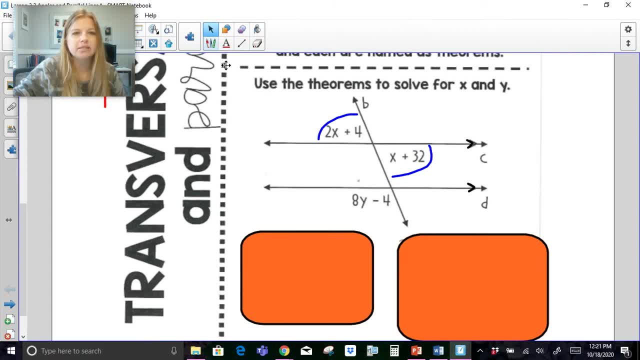 vertical angles And notice they both deal with the variable x. So I could go ahead and set those equal to each other, Solve for x, And because I have two x plus four, I can solve for x. And so what I'm going to do is I'm going to go ahead and make note that this is 28.. So I'm going to just go. 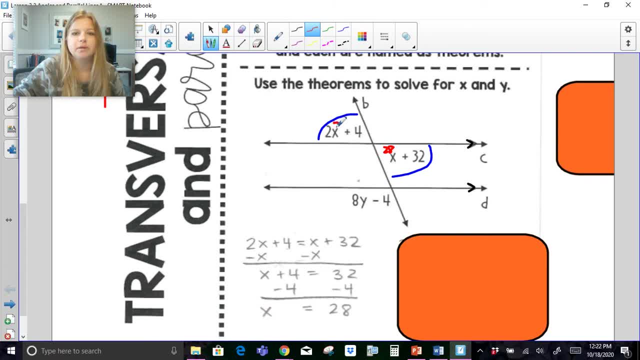 ahead and make note that this is 28.. Okay, x value is 28.. So now to figure out my y value. so let's think about this for a moment. If I know that this angle here is 28 plus 32,, this entire angle here. 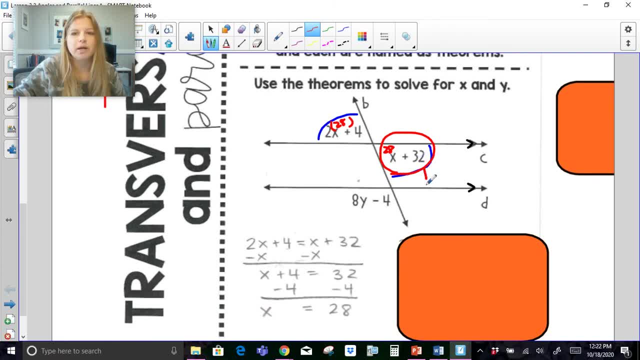 is 28 plus 32.. Well, that angle corresponds to this angle here. So this angle must also be 28 plus 32.. And if that angle is worth 28 plus 32, and these all together would add up to 180,. 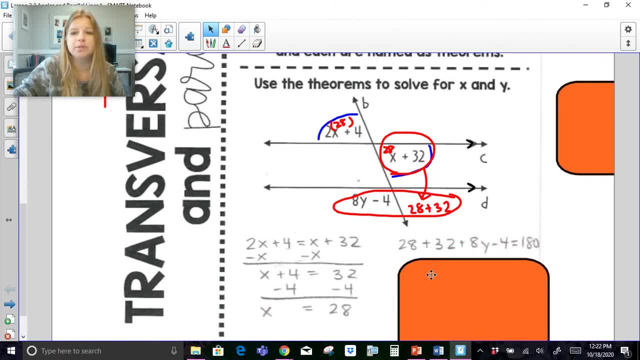 because they make a linear pair. that's what I could do. to end up solving for y, I could say that this angle here of 28 plus 32, plus this angle should add up to 180.. And then use my equation solving skills to get the answer. The other thing that I could do is I could figure: 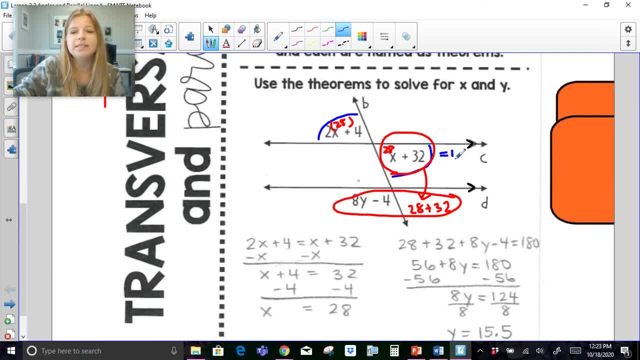 out: well, hey, 28 plus 32.. Let's see that: 60 degrees. So I could figure out: well, hey, 28 plus 32.. So I could figure out: well, hey, 28 plus 32.. Let's see that: 60 degrees. So if this is 60,. 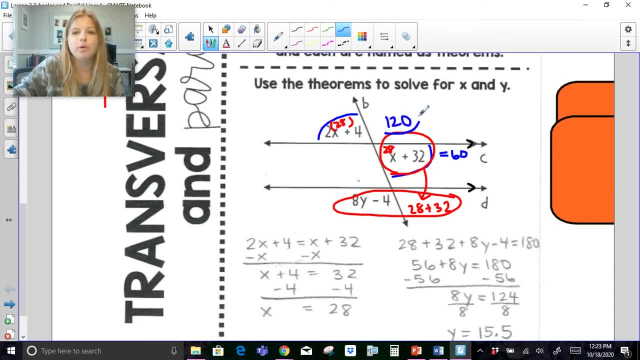 then this would have to be 120. And 120 would then have to be equal to 8y minus 4, because they are alternate exterior. So you definitely have a bunch of options of things you can do in order to solve. You just have to make sure you're using an appropriate theorem or a postulate that we 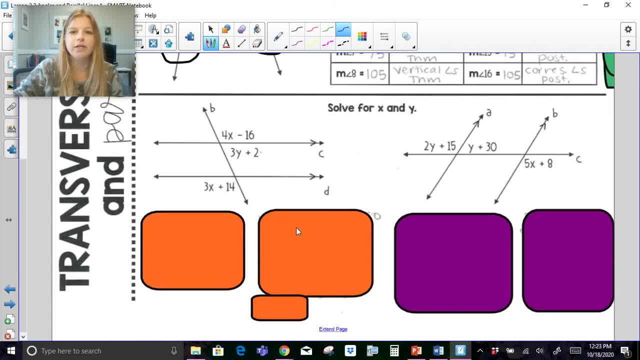 have been learning. So the same thing would go for here. solve for x and y. So I have to look at what I know for a fact I can solve. Remember, when you're solving a quick equation, you're setting up equations and we're not using any systems here. We don't really want. 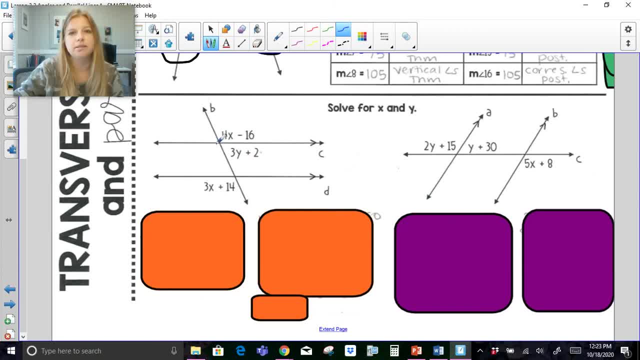 to mix and match. So we want to match up our x's and then see what we're left with. So this angle here of 4x minus 16 should be equal to 3x plus 14.. Those angles should be equal because they are. 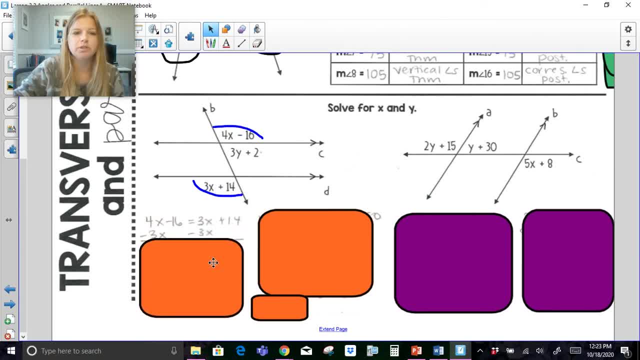 alternate exterior, So I can go ahead, set those equal to each other. solve my equation and get x equals 30 as my result. Then think about what's the relationship between the value I get for here after I substitute- and x is 30, and this angle here. Well, these angles form a linear pair. 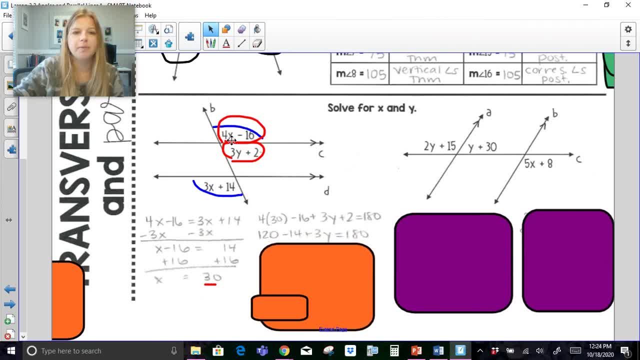 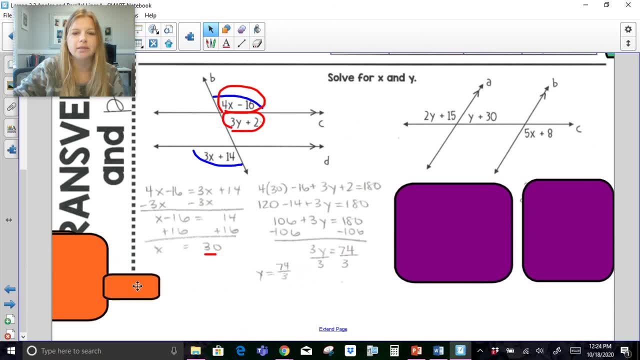 Linear pair are supplementary And so if I substitute in my 30 for x this angle plus this angle adds up to 180.. And just like the previous problem, I can go ahead and I can solve. Excuse me, Okay, last one here like this, So I have my relationship. 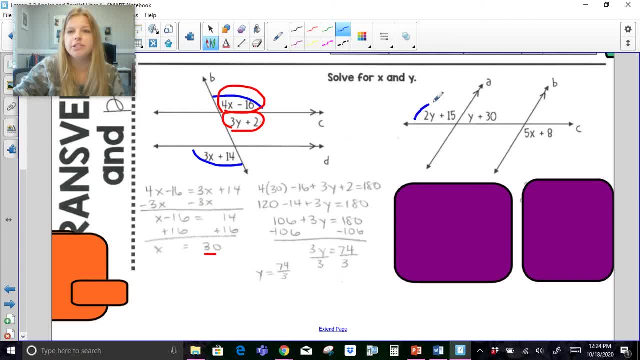 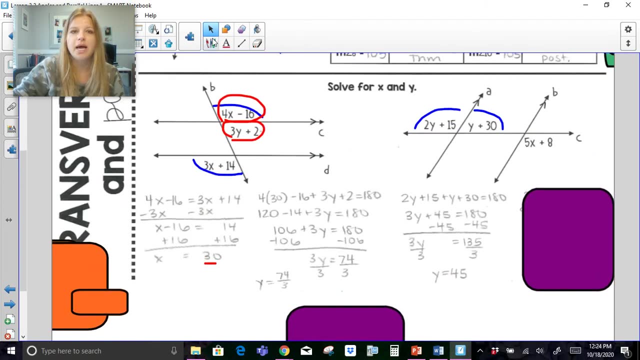 notice I have y's in two of these expressions, So I should be able to know that, okay, these two angles here would add up to 180, because they make a linear pair Be able to solve my equation. I get y equals 45. And then, once I know that y is equal to 45,, 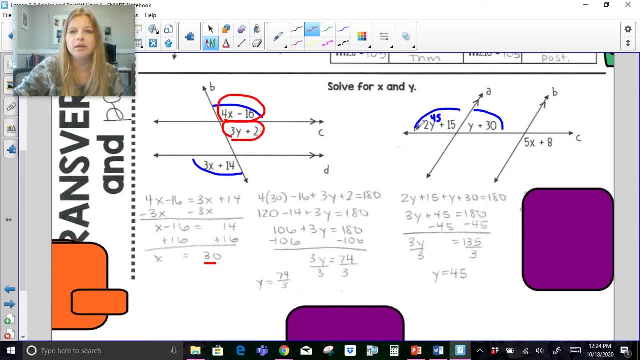 think about my relationship with these angles. in this angle here, This angle here and this angle here are alternate exterior, And if I substitute in my equation, I get y equals 45. And then, once I that means that they have equal measures for their angles, And so I would set them equal to each. 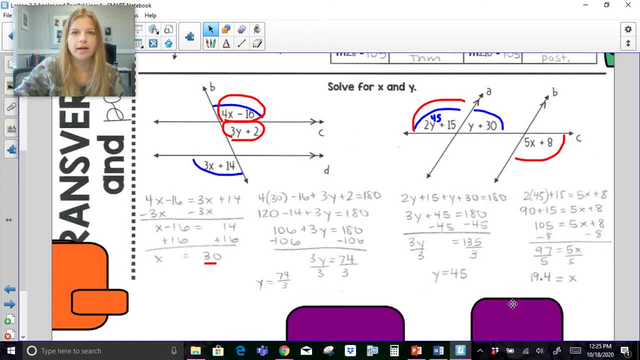 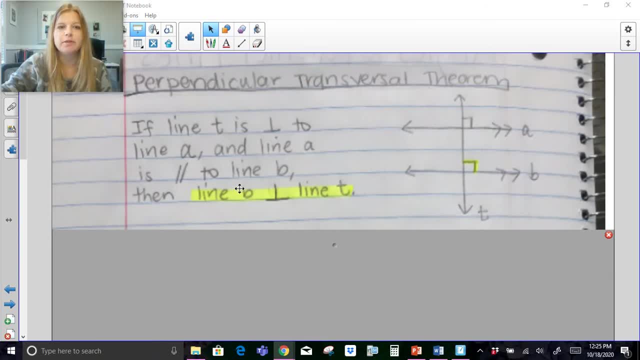 other, And then I would be able to solve for x. So again, we have to use what we know for a fact to be able to go forward. Now, the last part of this lesson is about the perpendicular transversal theorem. It says if line t- so here is line t- is perpendicular to line a, So let's 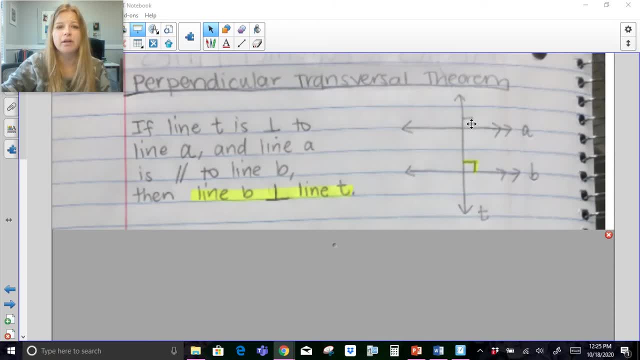 say, line t is perpendicular to line a- And you can see I have a little right angle marker there- And line a is parallel to line b. Well, that means that this line t is also perpendicular to line b. Okay, so it's basically saying, if I have two perpendicular lines and then this line here, 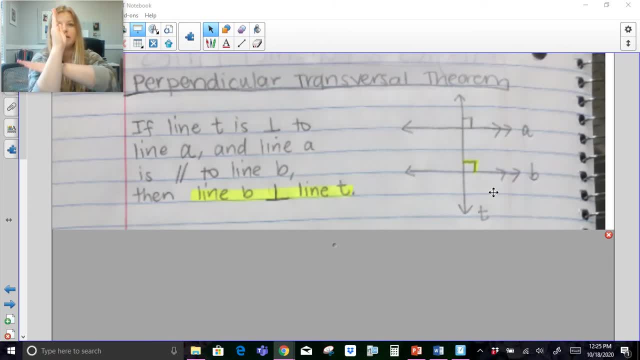 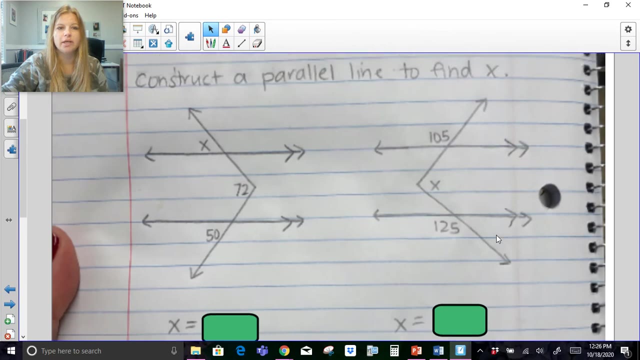 is parallel to this new line down here. if they're parallel- and I know one of them is perpendicular to this line- then that second line should also be perpendicular, And that is called the perpendicular transversal theorem. Now the last two kind of problems that we have to look at, say, ask us to solve for an angle here in the 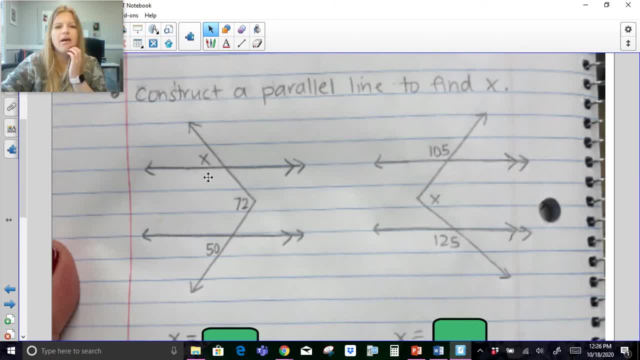 diagram where it looks kind of funky like what is even going on And we notice we have a set of parallel lines, but we need to figure out what this angle is And this angle has really no relationship directly with 50 or 72. It's kind of funky. So what it says here is: it says: construct a parallel line to find x. 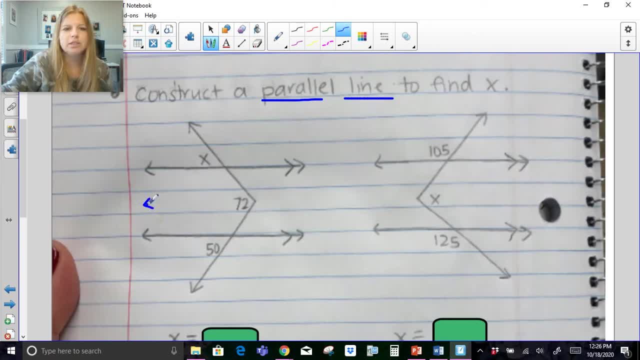 So when you have a diagram that looks like this, we would need to construct a new parallel line that actually goes directly through, where that kind of those two rays basically meet each other. Then we have to be able to fill in what we know for a fact. So I need to be able to get 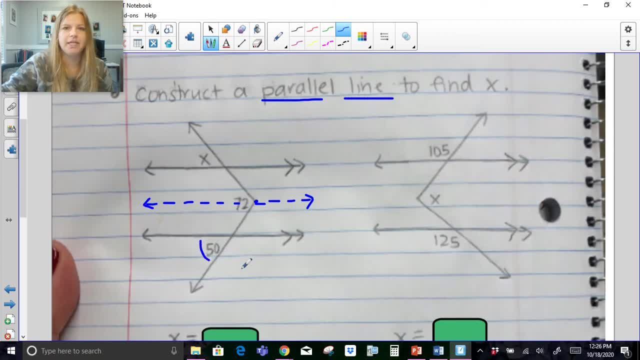 to angle x. This angle here is 50.. So by the vertical angles theorem I know this angle is also 50.. a new parallel line in between: if this is 50, then this little angle here is also 50, because those are alternate interiors. well, the entire angle here. 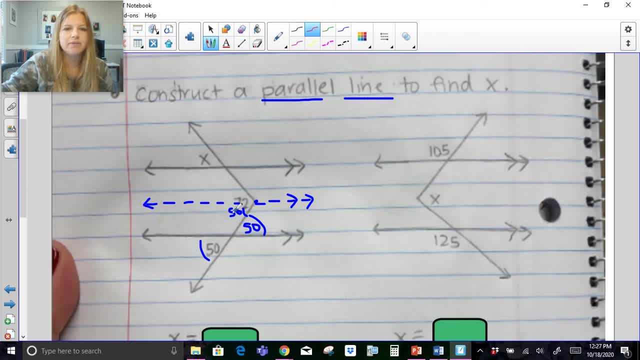 says it's 72. so let's see: if the entire angle here is 72 and this parts 50, that means that this part of the angle is worth 22, and if this part of the angle is worth 22, then these are what's called corresponding angles, and angle X is 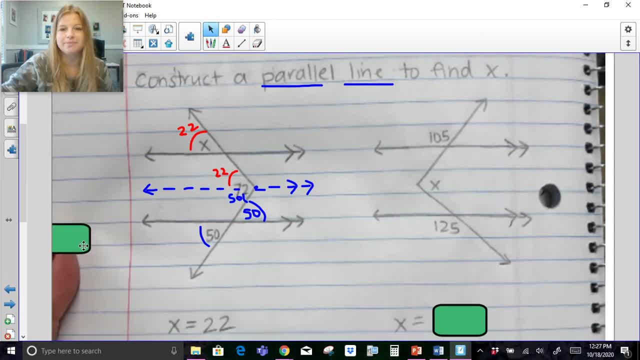 worth 20 is has a value of 22 degrees. let's try the same thing here. if I construct a perpendicular line- rather okay- to the other parallel line, so that a pair of three parallel lines- if this is 105, then this is 105, now these would. 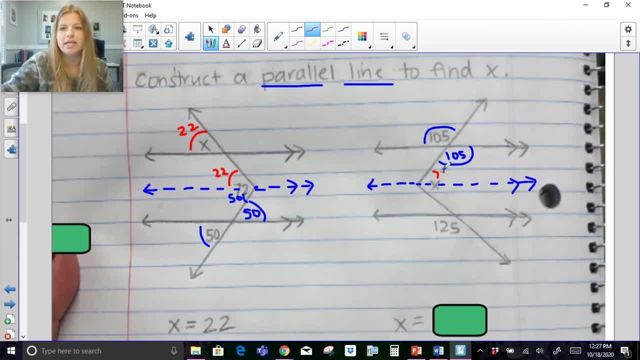 be alternate interior. so if this is 105, then this angle is 75 and that looks like it's part of X. but I need to figure out this segment, this part angle, right there. so if this is 125 and this is 125 because that's alternate, I'm 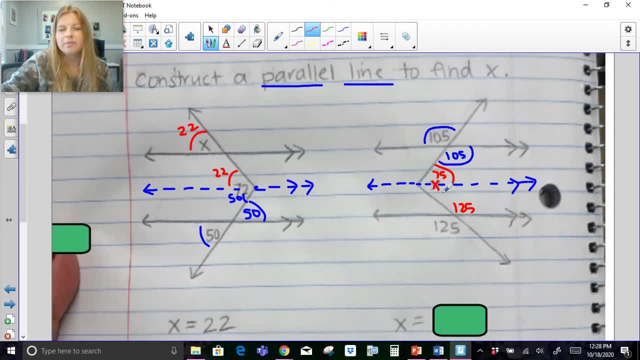 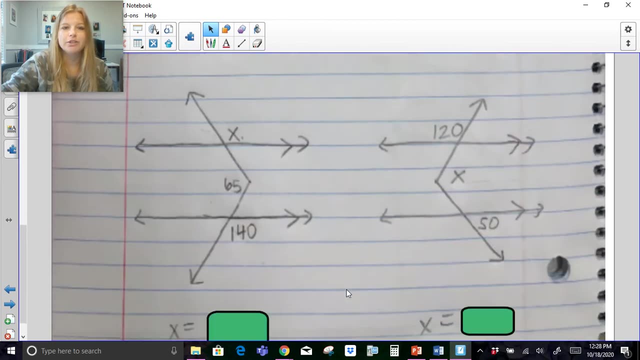 sorry, those are vertical angles. these would have to be consecutive interior. so if this is 125, then this angle is 55, and then I would simply add up 75 and 155 to get that X is equal to 130. you can try these last two problems on your own and 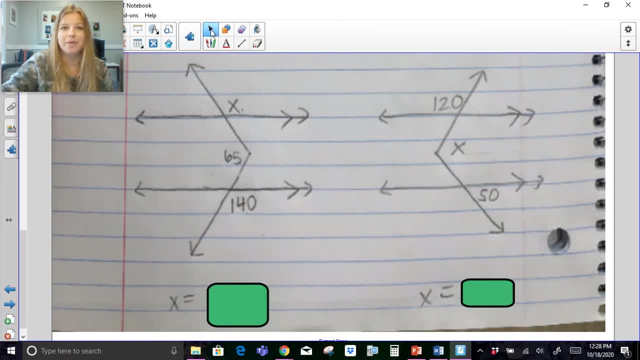 then press play to see if you can figure out what X should be. okay, let's take a look. if I construct my parallel line, if this is 140, then this is 140, which means that this little part of the angle is worth 40, if the entire. 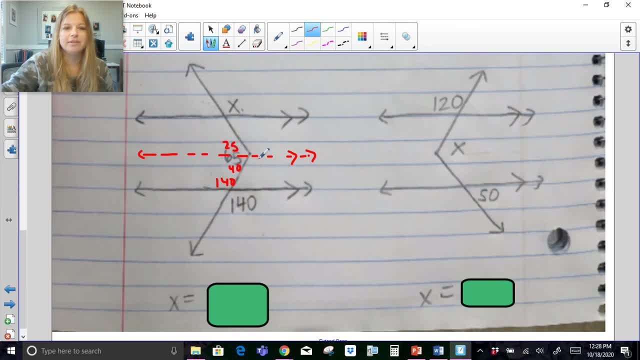 value is 65, then this has a value of 25. if this is 25, then this corresponds to this angle of 25, which means that my X value would have to be 155, because those are supplementary to each other. and then, for my last one, if I construct a parallel line, if this is 50, then this: 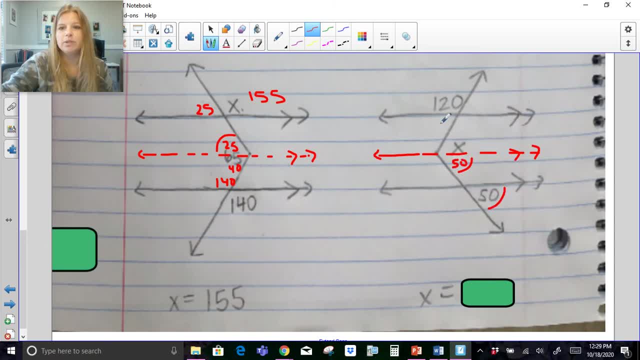 is 50 because those are corresponding angles. if this is 120, then this is 120 because those are corresponding, and if this is 120, then that means this angle here X is 60 because those are supplementary, so the entire value of X would be 60 plus 50, which is 110. thank you so much for watching this video. I 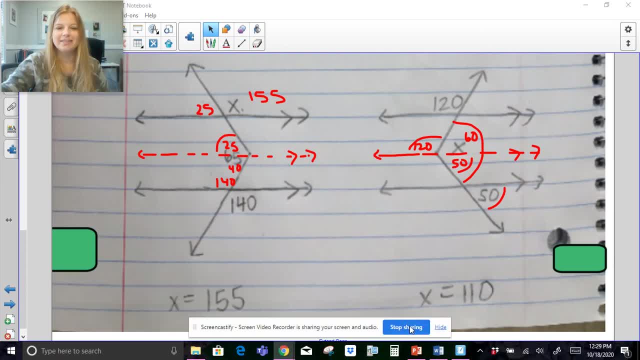 hope it was helpful bye you.